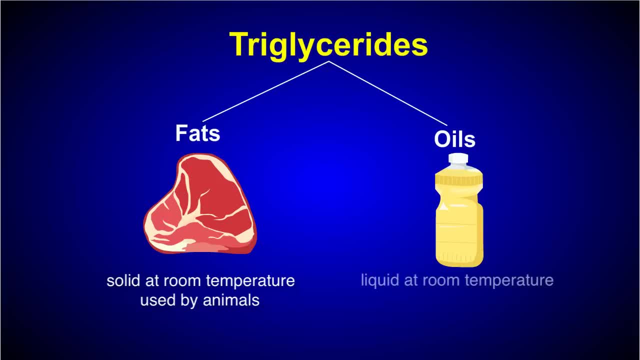 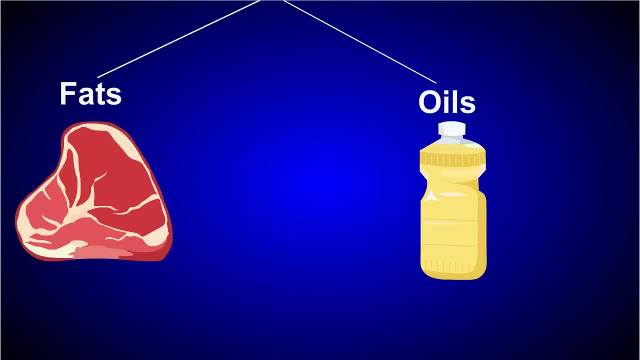 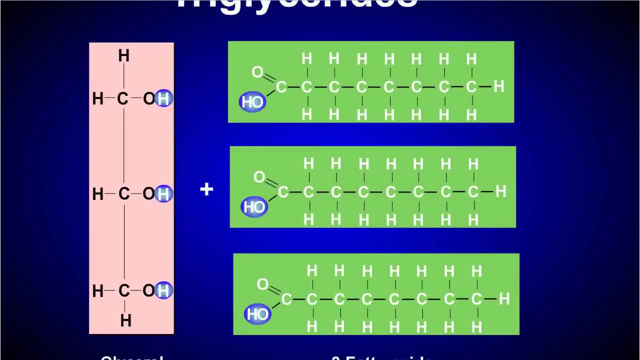 Oils such as corn oil and olive oil are liquid at room temperature and are used by plants for long-term energy storage. At the molecular level, triglycerides contain two types of subunit molecules: Glycerol and fatty acids. Let's take a quick look at fatty acids. 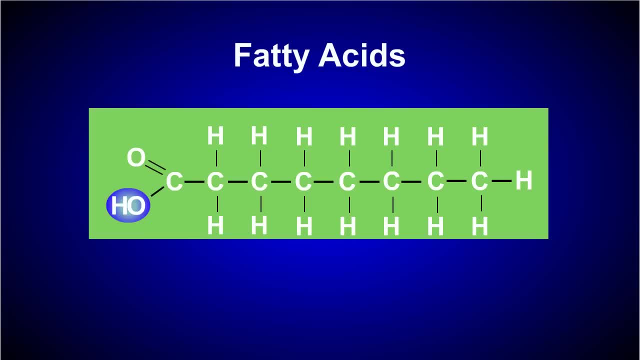 A fatty acid has three main parts: a chain of carbon and hydrogen atoms called the hydrocarbon chain, a methyl group at one end and an acid group at the other end. Fatty acids can either be saturated or unsaturated. A fatty acid that has only single carbon-to-carbon bonds is known. 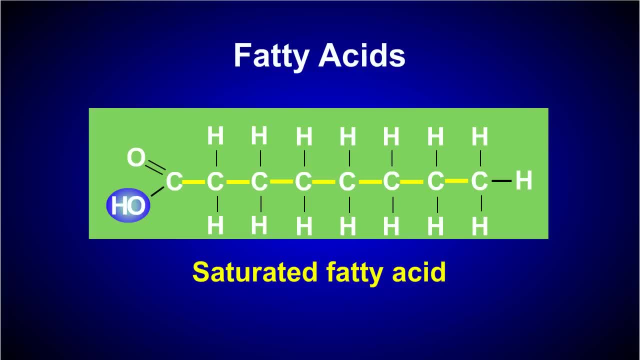 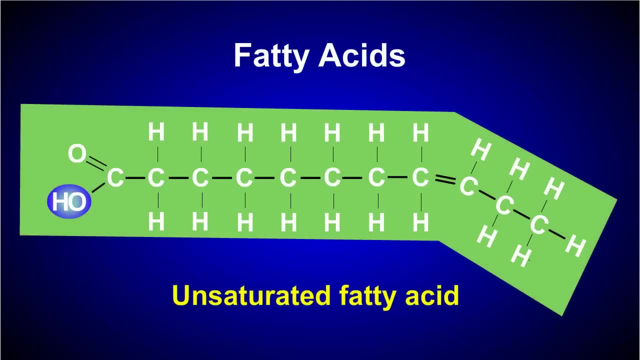 as a saturated fatty acid. This is because the carbon chain is saturated with all the hydrogen atoms it can hold. Unsaturated fatty acids have one to several double bonds. Double bonds result in kinks in the fatty acid chain, which affects the melting point of the fat. 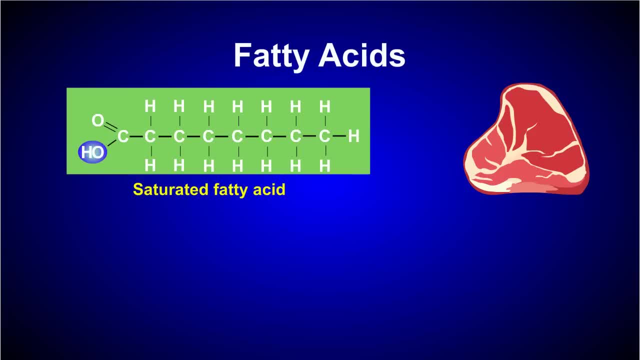 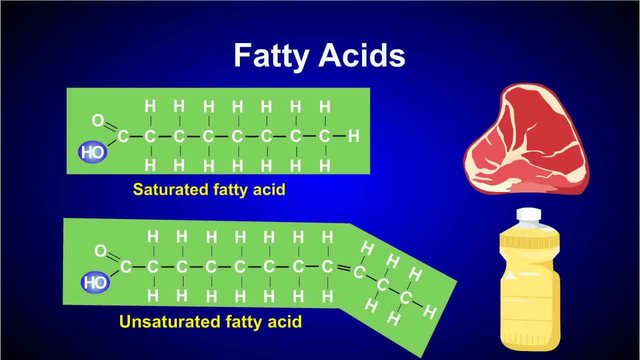 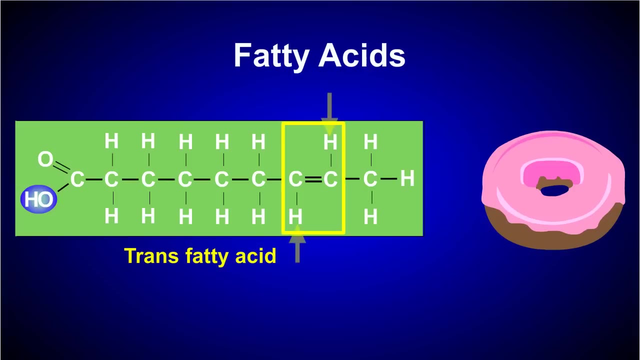 Animal fats have saturated fatty acids and are solid at room temperature, while vegetable oils have one or more double bonds and are liquid at room temperature. A trans fat is an example of an unsaturated fatty acid, where the hydrogen atoms are on opposite sides of the double bond. 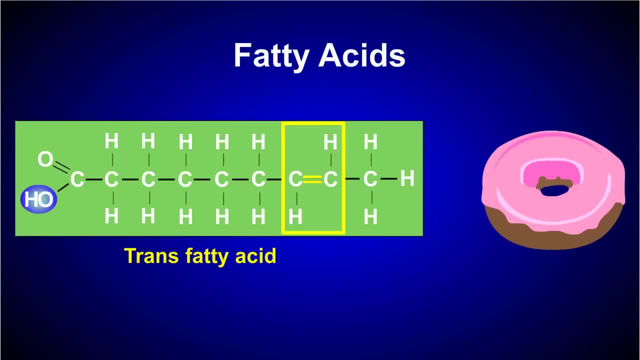 Trans fats are usually formed during the production of processed foods and are also commonly in partially hydrogenated oils. In order to increase shelf life and melting point of the fat, excess hydrogen atoms are introduced to an unsaturated oil. This causes the formation of trans fat bonds in the fatty acid chain. 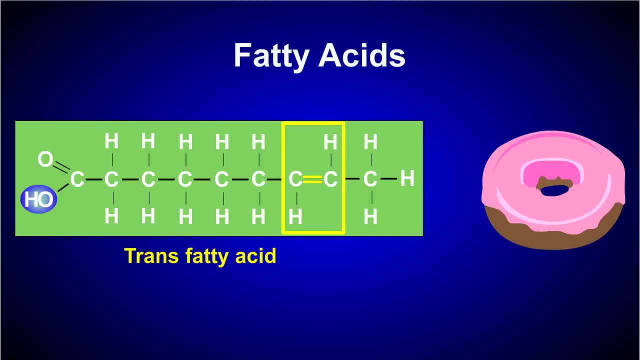 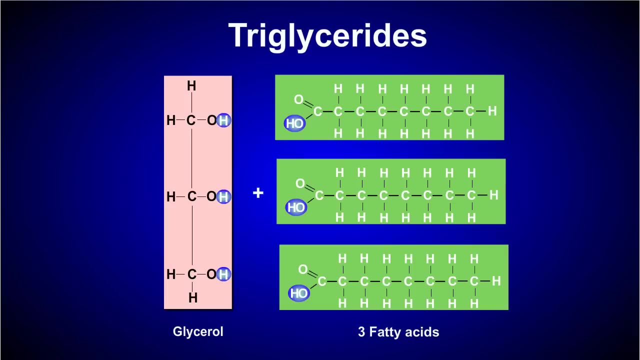 Unfortunately, the consumption of trans fats has been associated with cardiovascular disease and its use has fallen from favor. Now that you understand a little bit about fatty acids, let's zoom back out and look at how the triglyceride subunits fit together. Remember, a fatty acid is only a small part of a triglyceride. 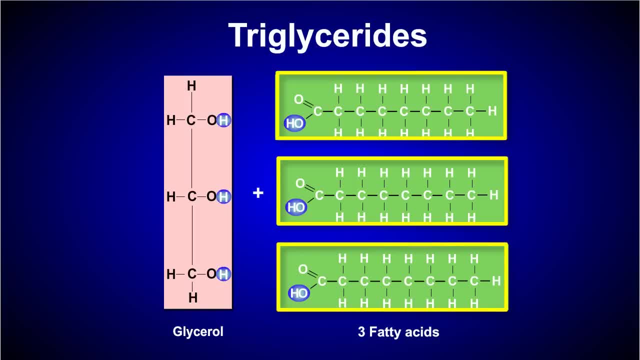 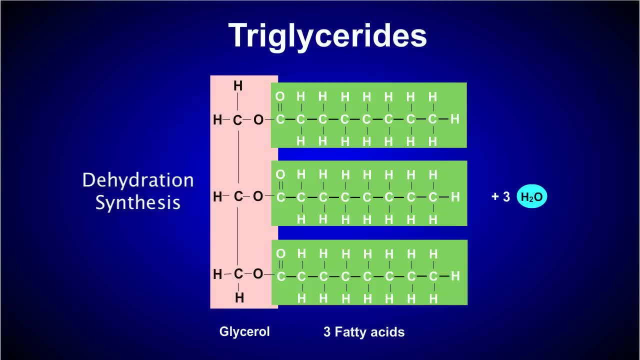 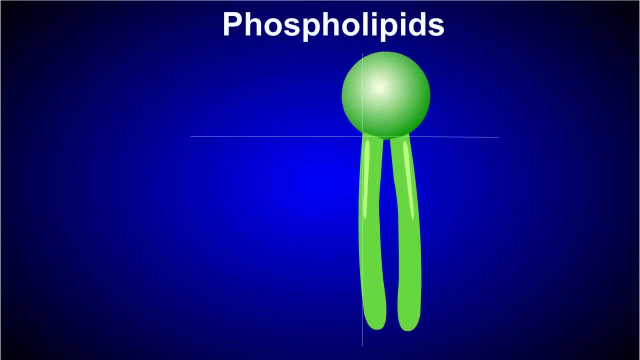 To become a triglyceride, three separate fatty acids have to bond with a glycerol molecule through the process of dehydration synthesis. Let's move on to the next category of lipids, which is phospholipids. Phospholipids are similar to triglycerides in that they contain glycerol and two fatty acids. 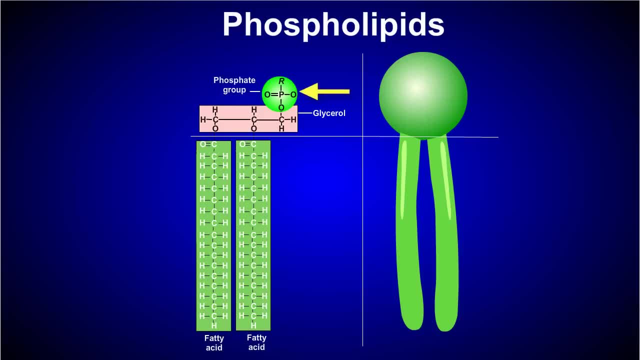 What's different is that a phosphate group, rather than a third fatty acid, is attached to the third carbon of glycerol. Phospholipids are extremely important, mainly because of their unique properties in regard to water. The phosphate head of the molecule is called the glycerol. 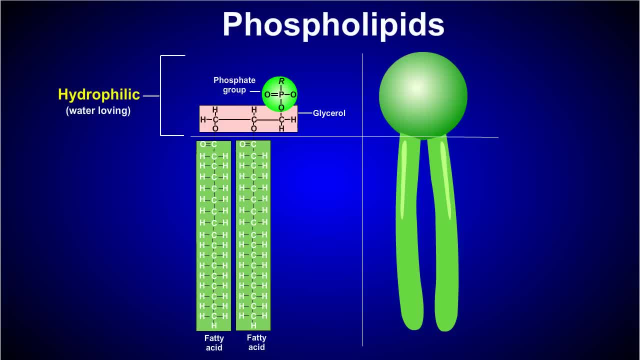 Phospholipids are extremely important, mainly because of their unique properties in regard to water. The phosphate head of the molecule is called the glycerol. This structure is hydrophilic or water-loving. This means that it mixes well with water. 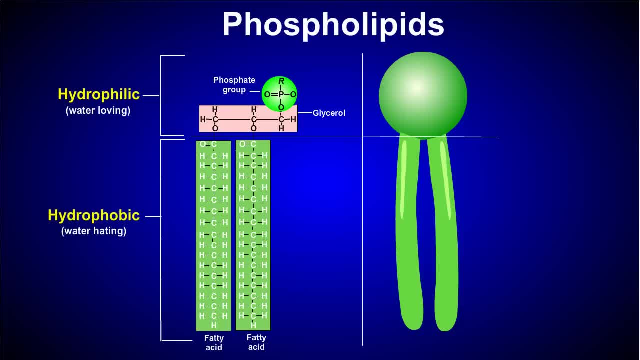 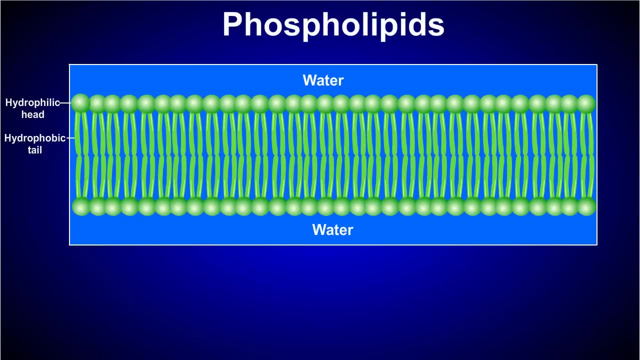 The fatty acid tails, however, are hydrophobic or water-heating and do not mix well with water. Because of these unique properties, phospholipids tend to arrange themselves so that only the hydrophilic heads interact with the watery environment and the hydrophobic tails crowd. 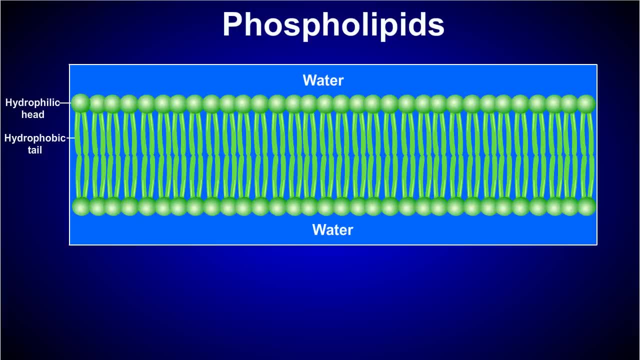 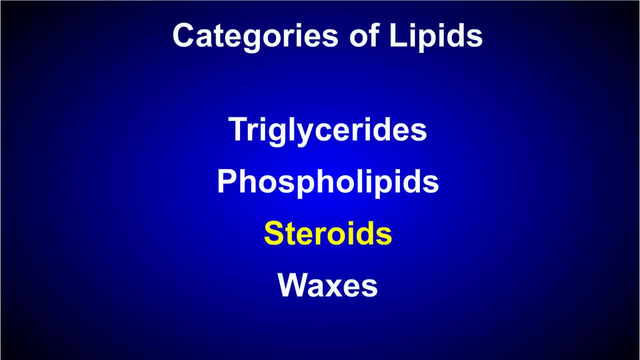 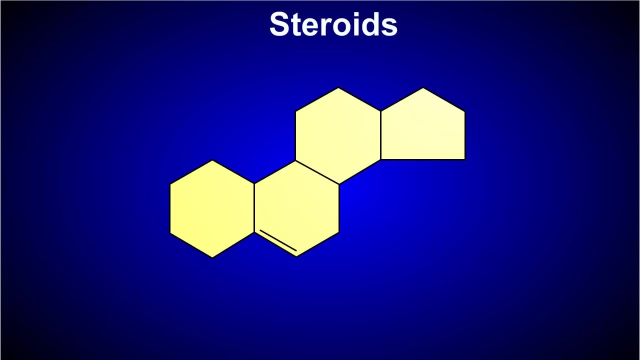 inward, away from the water. áthis structure is the major component of plasma membranes of the cell. Steroids are the next category of lipids. Steroids are composed of four fused rings of carbon to which different functional groups are attached. One well-known steroid molecule is cholesterol. 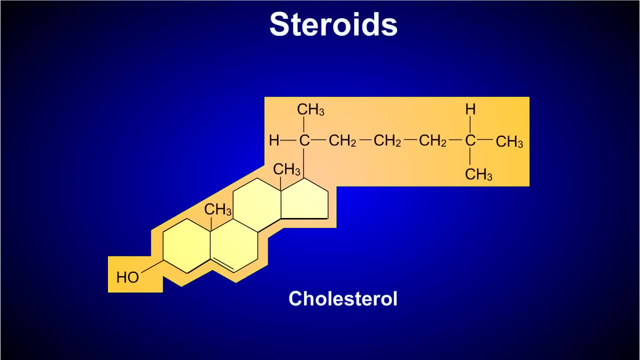 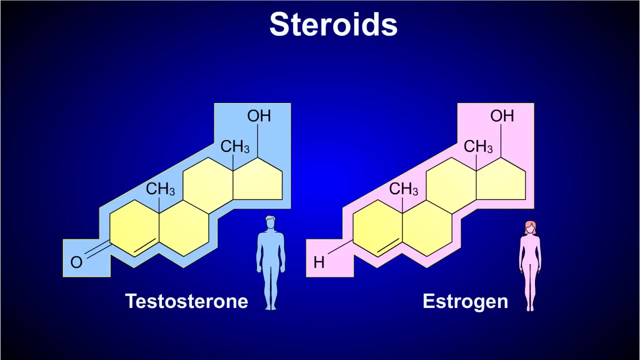 Cholesterol serves as a precursor for the synthesis of other steroids such as testosterone, estrogen, vitamin D and cortisone. Cholesterol is present in plasma membranes, where it stabilizes the membrane. The hormones testosterone and estrogen have small differences in their functional groups. 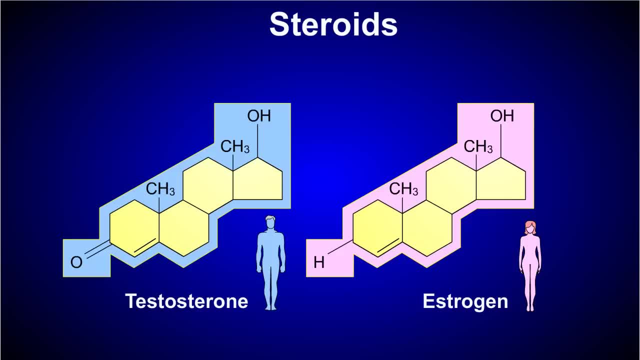 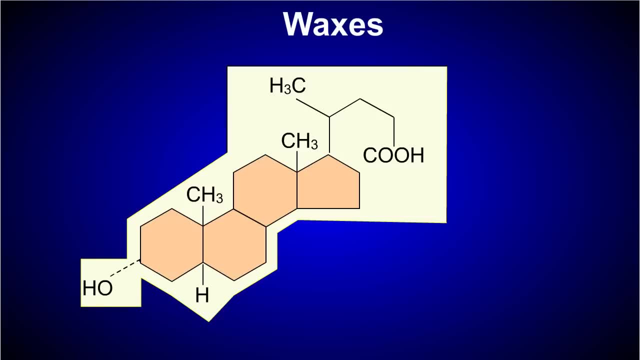 but large differences in their effects on an organism. Waxes are the final group of lipids. Waxes are non-polar and repel water. They're found in the protective coating on leaves and on outer surfaces of animals. Waxes produce in the ears of some animals to protect the eardrum. 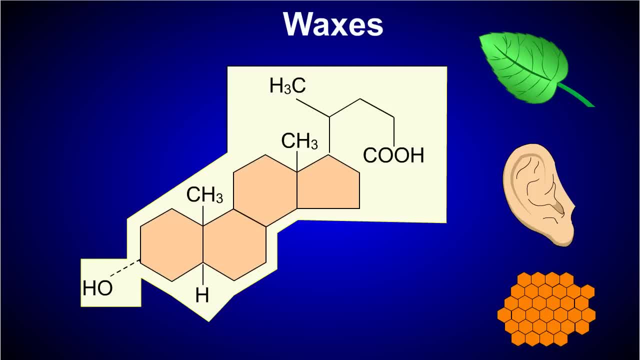 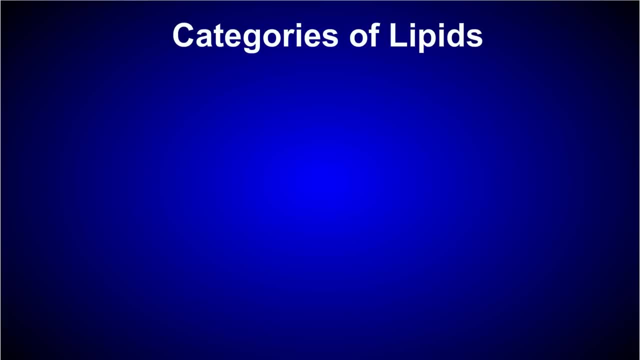 In addition, bees construct honeycombs from wax. Now that we've covered all four categories of lipids, let's do a quick recap. The four categories of lipids are triglycerides, phospholipids, steroids and waxes. 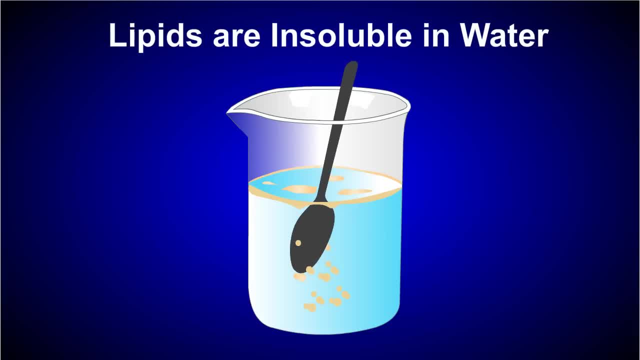 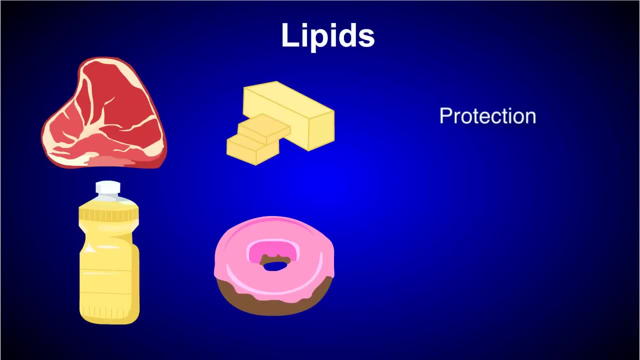 All lipids are insoluble in water. While the primary function of lipids is long-term energy storage, lipids are also used for a multitude of other purposes, such as protection and insulation, and as a key component of hormones and cell membranes.